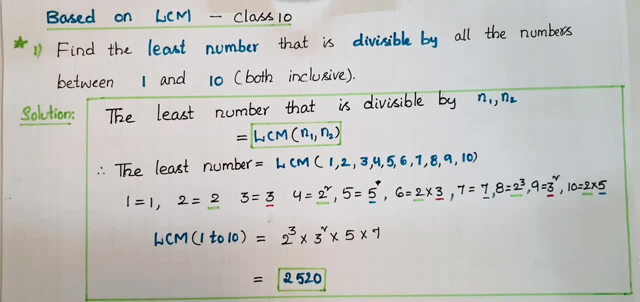 Hello everyone. today I am going to tell the problems which are based on LCM. The first one is: find the least number that is divisible by all the numbers between 1 and 10, both inclusive. So that means it includes 1 and 10 also. So we know that the least number that is divisible by any two. 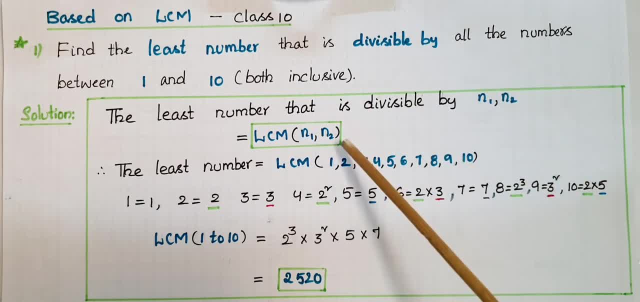 numbers n1 comma n2 is equal to LCM of n1 comma n2.. So here we have to find LCM of these numbers, 1 to 10 numbers. So for that we have to prime factorize these numbers first. So 1 is equal to. 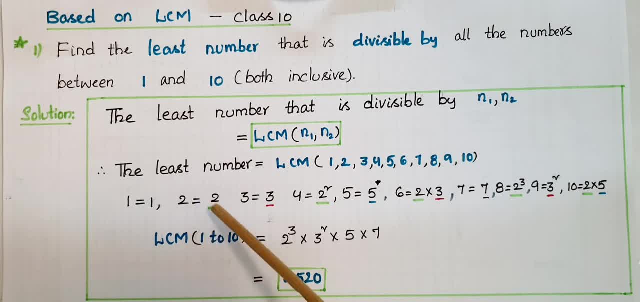 1,. you can factorize like this: 2 is equal to 2, 2 is a prime factor, So 2 is equal to 2, 3 is equal to 3 and 4 we can express as 2 square, and 5 we can express as 5, 6 we can express as 2 into 3. 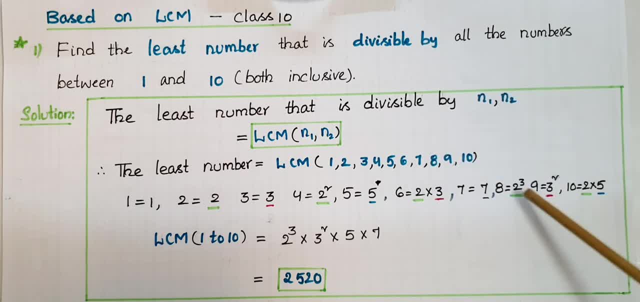 and 7 is equal to 7 and 8 is equal to 2 cube, 9 is equal to 3 square and 10 is equal to 2 into 5.. So we have to find LCM from 1 to 10 numbers, So including 1 and 10.. So that is first to see the 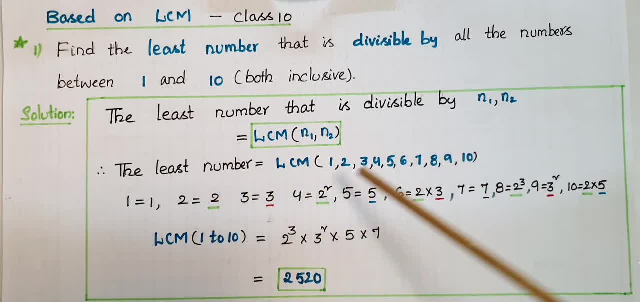 common factors here. So here 2 is common and see the highest power also 2 is common and highest power is here 2 cube. So 2 cube into for 3, here 3 and 3 and 3 square. highest power is 3 square. So into 3 square. 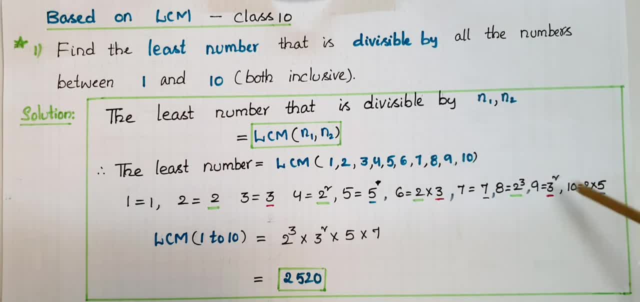 into again 5.. So here also 5.. So 5 into 7.. So write 7 here. So there are no other numbers except 1. So these are the common factors and other numbers also only 1. So multiply these numbers. 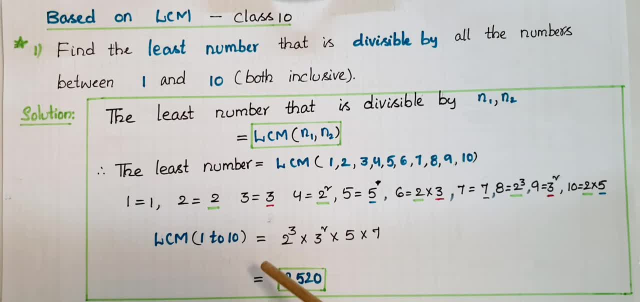 then you will get 2520.. This is LCM of all the numbers between 1 to 10, including 1 and 10.. Now we can check whether this LCM is divisible by all the numbers from 1 to 10, including 1 and 10.. 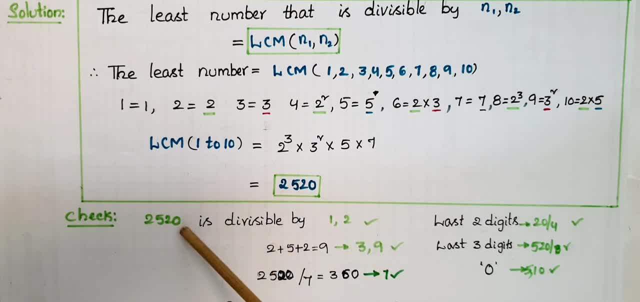 So it is divisible by 1 and 2, because last digit is 0 and last 2 digits are 2 and 0. So that is divisible by 4 and last 3 digits divisible by 8. So this is divisible by 8.. This number is divisible.